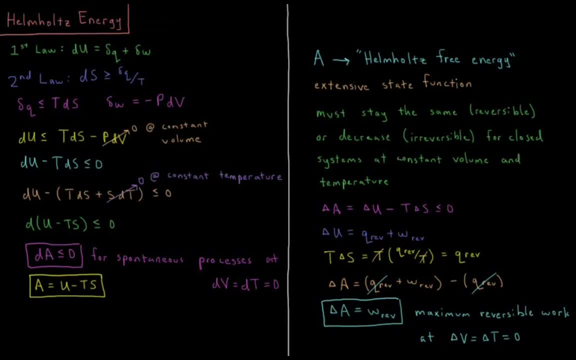 This video will discuss the Helmholtz energy in chemical thermodynamics. So from the first law of thermodynamics we saw that the energy change of an isolated system during any physical process is equal to zero, And for a closed system it has to. 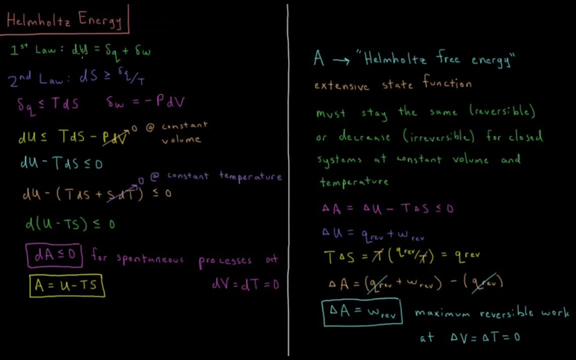 be matched by the energy change of the surroundings. So du, for a closed system, the change in the internal energy during some physical process is going to be the heat dq plus the work. dw. inexact differentials for heat and work because those are path functions, exact differentials. 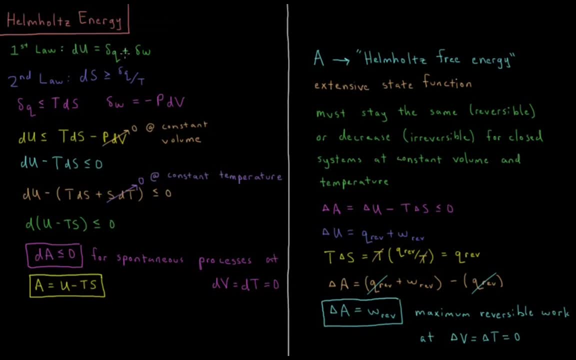 for du, because that is a state function. So we can either absorb energy into the system or release it as heat, or we can take in energy or release it as mechanical work. Specifically, the only type of work we're interested in right now is the energy change in the internal energy. So we can either absorb energy into the system or release it as heat, or we can take in energy or release it as mechanical work. Specifically, the only type of work we're interested in right now is the energy change in the internal. 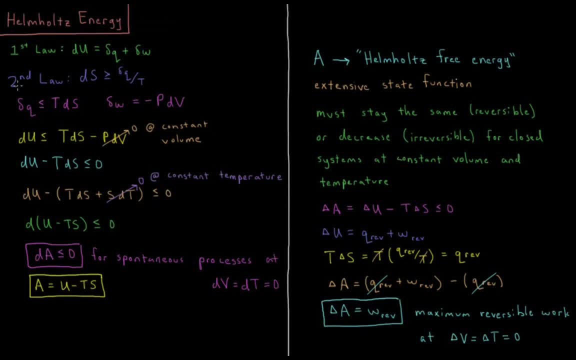 mechanical pressure volume work. Then the second law of thermodynamics says that for any physical process that occurs in an isolated system that the entropy change ds is greater than or equal to the change in heat. so dq divided by temperature. So rearranging these, 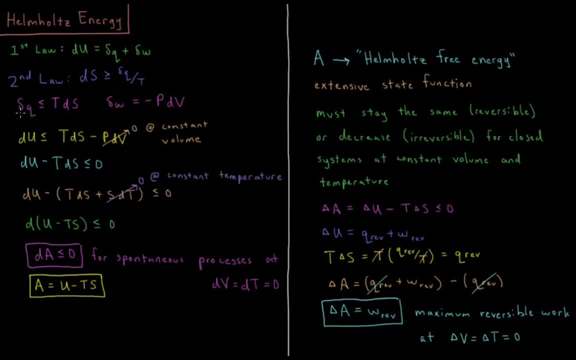 for heat and work. we have that the heat that occurs during some infinitesimal change in change in the system is going to be less than or equal to the temperature times, the change in entropy, TdS And the amount of work that occurs during that small system perturbation is equal to. 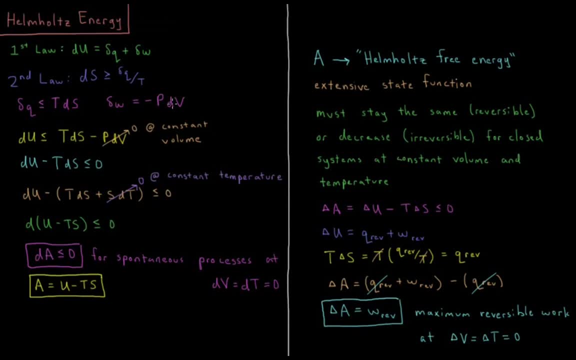 minus PdV. pressure times change in volume. So putting those two together, du is dq plus dw. dq is less than or equal to TdS, dw is equal to minus PdV. du change in internal energy is going to be less than or equal to TdS minus PdV. Now let's consider that this process occurs. 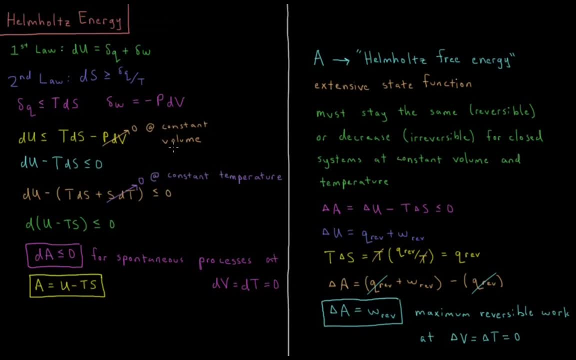 at a constant volume. So whatever process of interest is going to be at a constant volume. So now du is less than or equal to TdS, or du minus TdS is less than or equal to zero. So we can also say, if we make the following claim, that du minus the quantity, TdS plus SdT is: 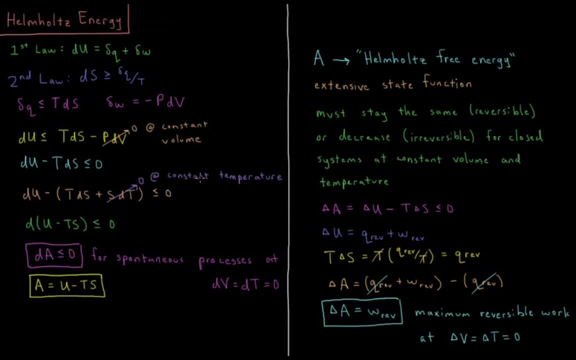 less than or equal to zero if this occurs at a constant temperature as well, Because dT would be zero and dV would be zero if we're at a constant temperature and volume. So TdS plus SdT is d of the quantity Tf. So we can also say that du minus TdS plus SdT is less than or equal to zero. So 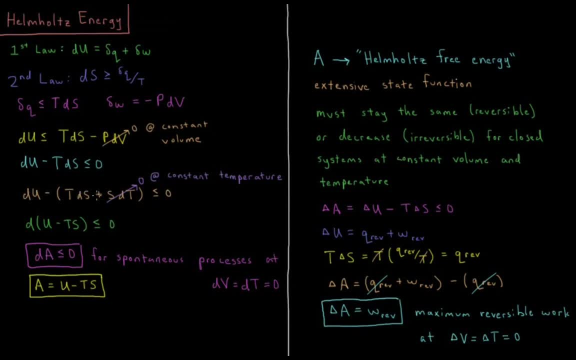 we can also say that du minus TdS minus SdT is less than or equal to zero. So this whole quantity is d of the quantity u minus Ts. So du minus Ts is less than or equal to zero according to the first two laws of thermodynamics. if we have a process which occurs at a constant temperature, 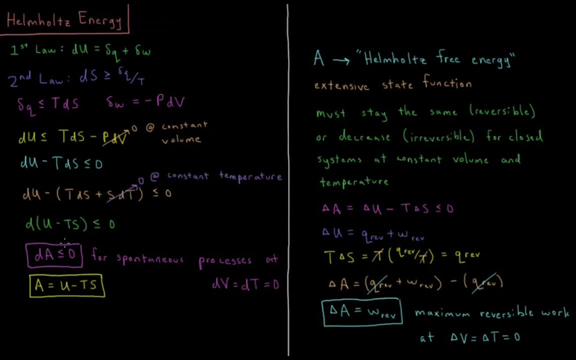 and a constant volume. So what we're going to do is we're going to define a quantity called A, and A is equal to the internal energy u minus the temperature times, the entropy of the system, Ts, And for a spontaneous process at: 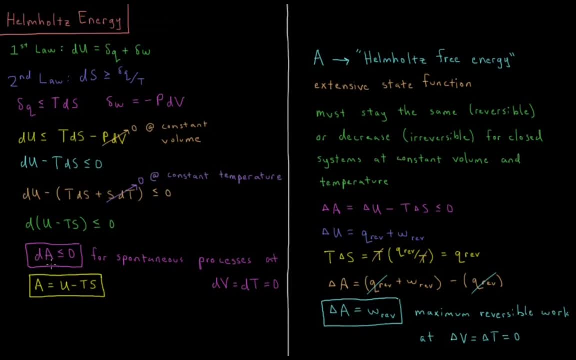 constant volume and constant temperature, the change in A is going to be less than or equal to zero. So what is this quantity here? A? We're going to define this quantity A as the Helmholtz free energy, Helmholtz being the name of the scientist who came up with this idea. So the 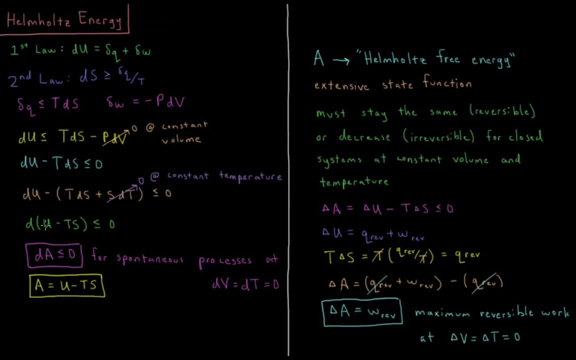 Helmholtz free energy, just like the entropy and just like the internal energy, is going to be an extensive state function. So the Helmholtz free energy must stay the same if a process is reversible, or decrease if a process is irreversible for closed systems at constant volume. and